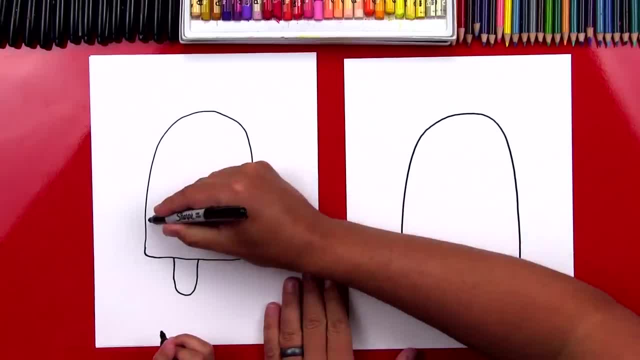 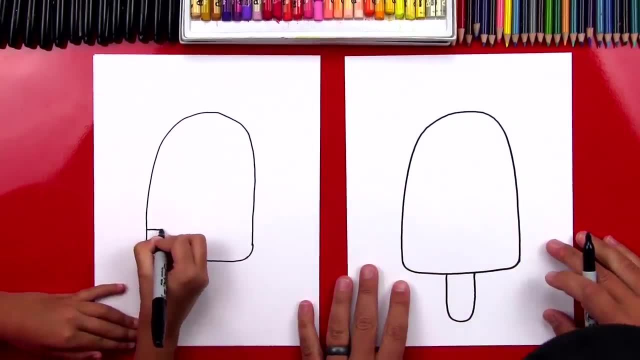 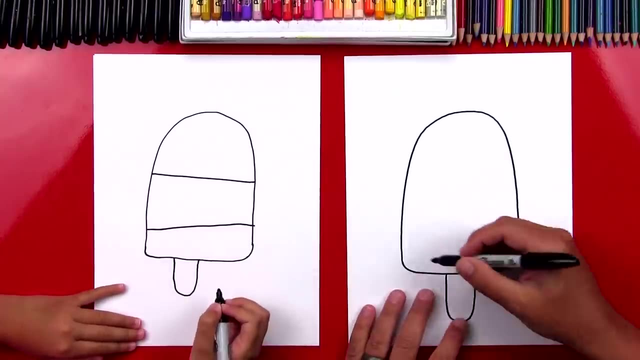 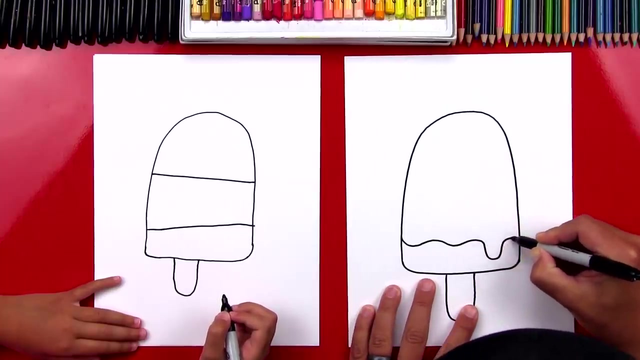 Okay, Okay. So first let's draw your stripes, And we're going to draw one stripe that goes across here and another stripe up here, So you have three stripes. Okay, Good, Now I'm going to draw mine dipped. So I'm going to start down here and I'm going to draw a wavy line like this And then I'm going to draw another, like a bigger drip right there on the right. 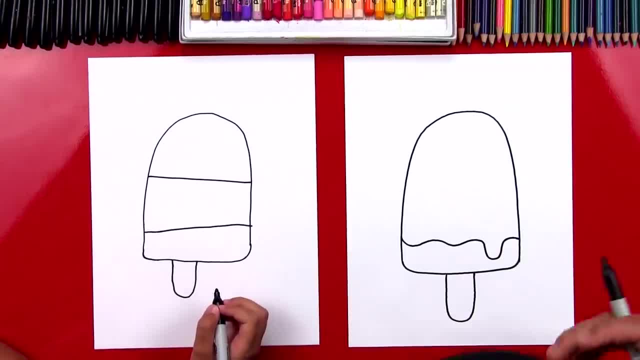 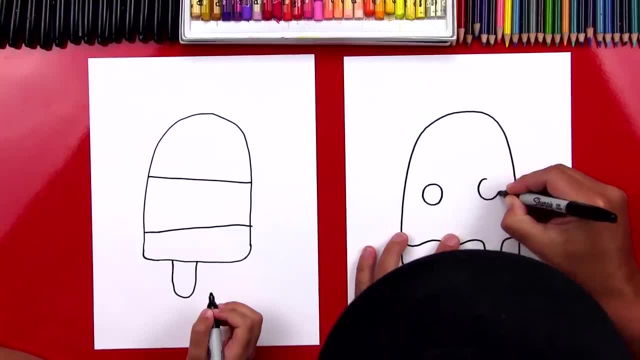 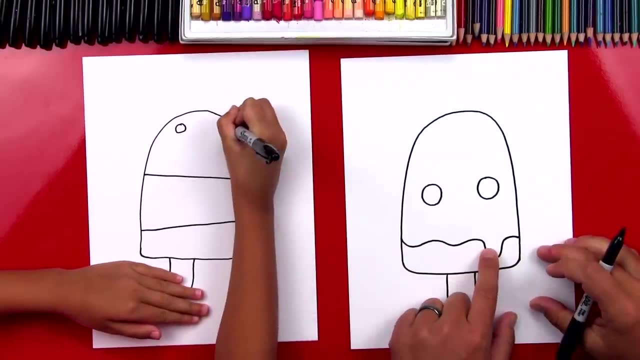 Mmm, Mmm. That looks really good, doesn't it? Now let's draw the funny face. So let's draw two circles. I'm going to draw one right here and one right here, And you can draw your funny face up here on the top stripe if you want. It kind of looks like he's grumpy, huh, And this is his eyes. this is his mouth. 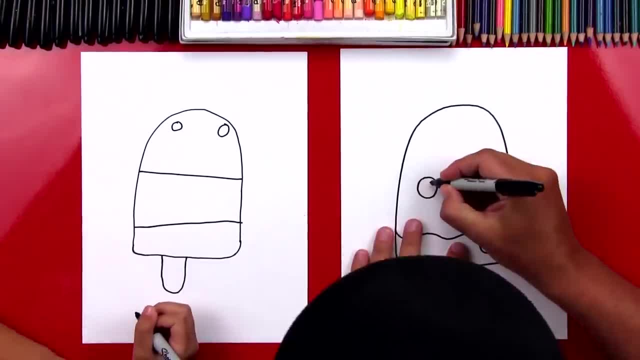 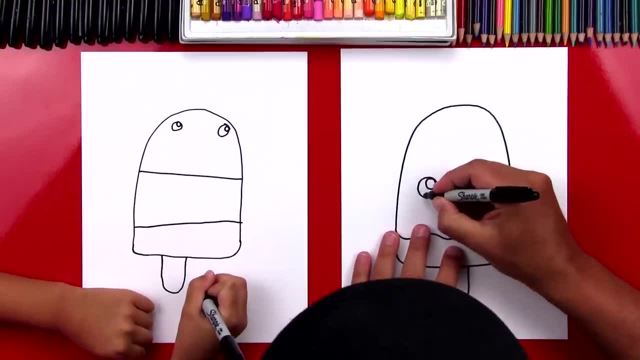 Okay, Okay. Okay Now, inside, let's draw a smaller circle in the top right And I'm going to draw an even smaller circle down here at the bottom, And you can leave that off, since your eyes are a little bit smaller. 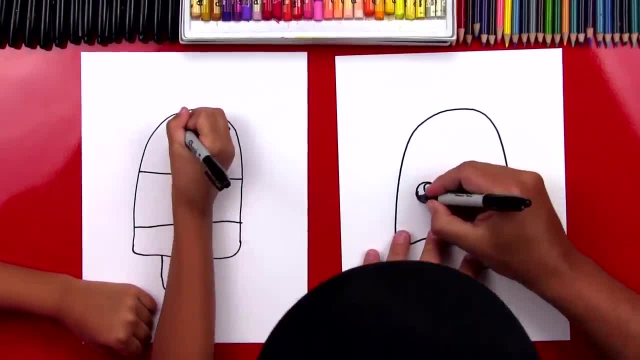 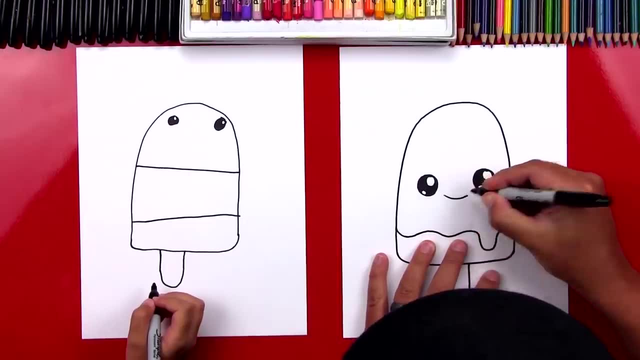 Mm-hmm. And then let's color in the big circle, but leave the little circles white. Okay, Next let's draw a cartoon mouth. I'm going to draw, I'm going to draw a happy mouth like this, right in between the eyes. 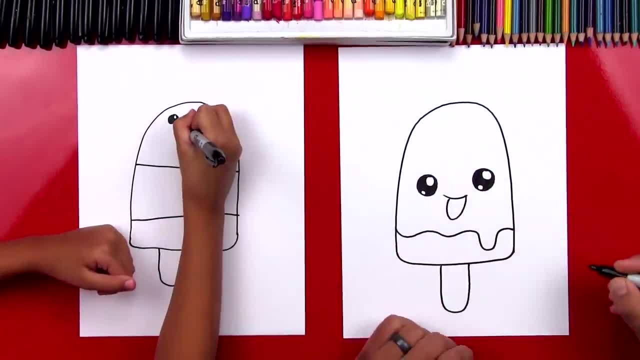 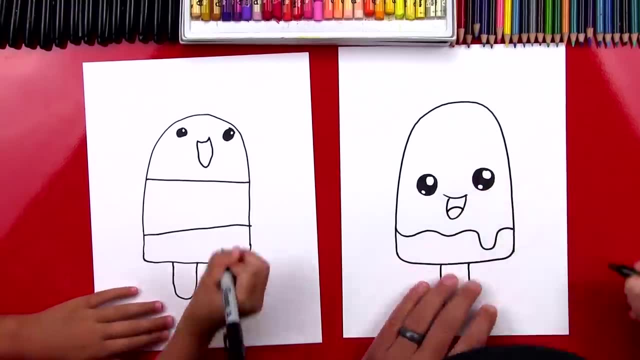 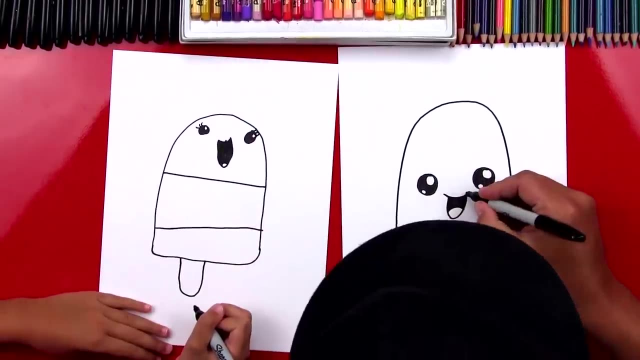 And then I'm also going to draw it, so it's open, Okay, And then inside, inside of our popsicle's mouth, I'm going to do a little rainbow line for her tongue, and then we can color in the top part. Okay, Next I'm going to add a little cheek line right here on the side. 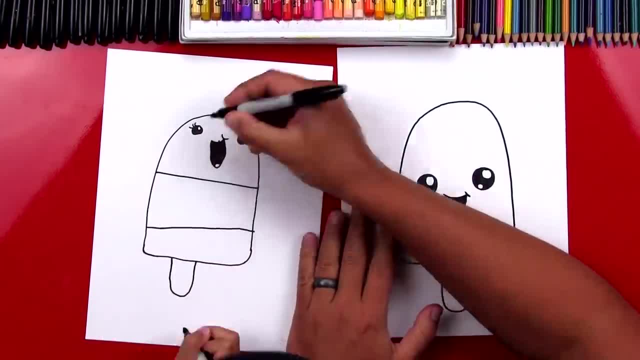 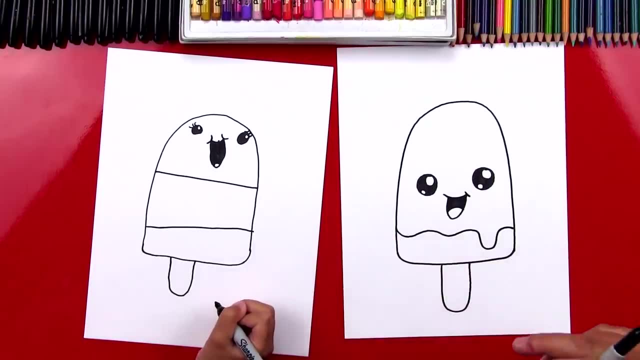 And we did it. You know you could add another one on the other side. Yes, That's my favorite little cartoon face I've ever seen. All right, We finished our popsicles. They look awesome and I love that they're different. 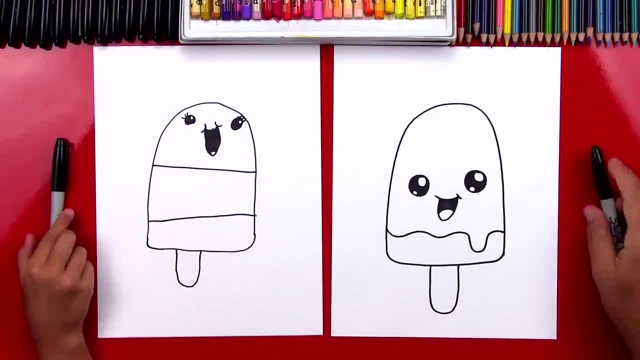 We used our creativity to change them and to make them our own. Now we still need to do one last thing, right? Yes, What do we need to do? Color, Okay, On the count of three, let's color them. 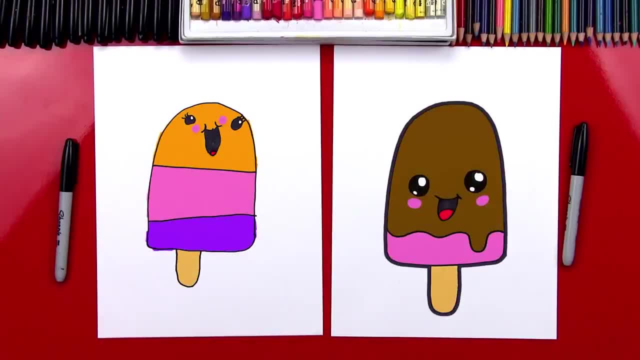 One, two, three. Oh wow, Nice job Hads You colored yours orange, pink and Purple. Purple, Mine's strawberry flavor dipped in chocolate. Mm-hmm, Oh tasty. Can you taste it?